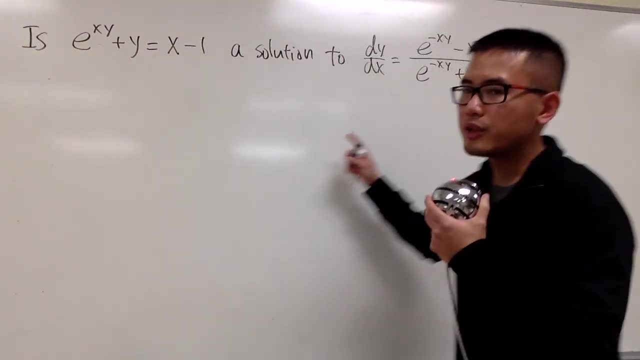 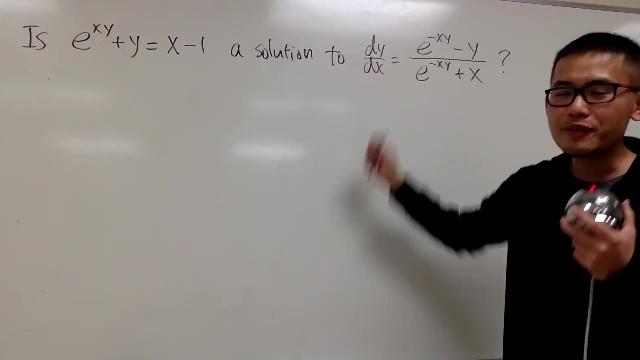 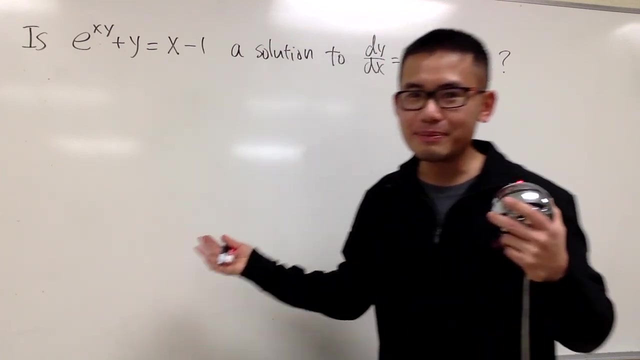 Okay, we are going to check if this equation is a solution to this differential equation. And this is technically a differential equation because we have a derivative right And the equation has a derivative. that is a differential equation. Anyways, right here to get the derivative of this equation. the y is not isolated. but what can we do? 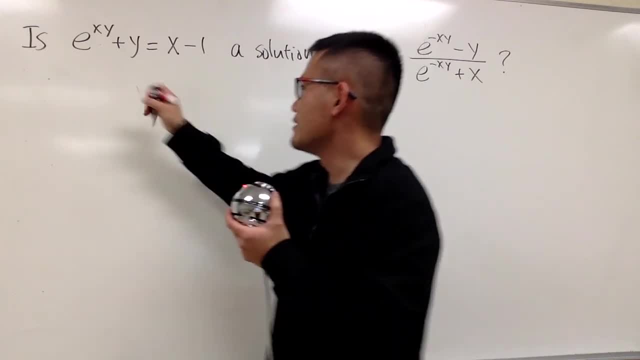 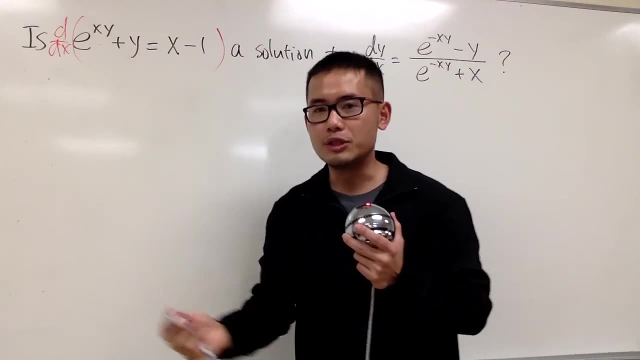 We can just use implicit differentiation, right? So it's okay, we can still do it and let's get to work. Let me put down d dx all the way in the front to show that we are going to differentiate this equation with respect to x. 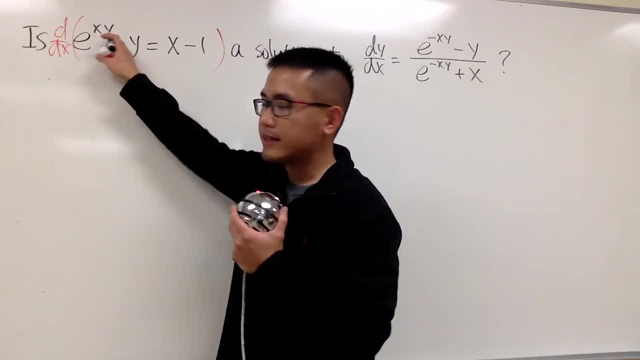 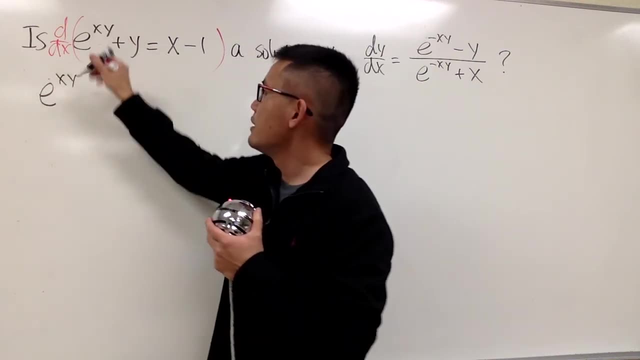 So let's get to work. First the derivative of e to the xy, the derivative of e to the something it is. first you repeat that it's just e to the xy right, And the chain rule says we have to multiply by the derivative of the inside. 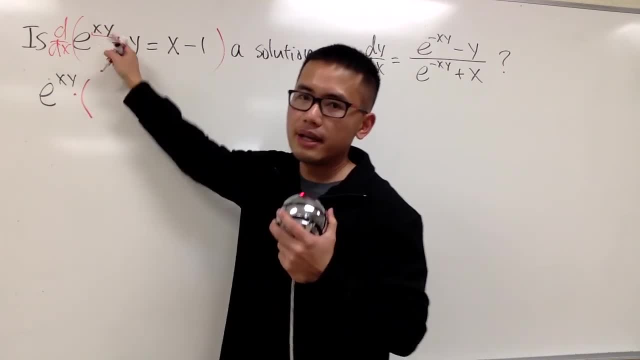 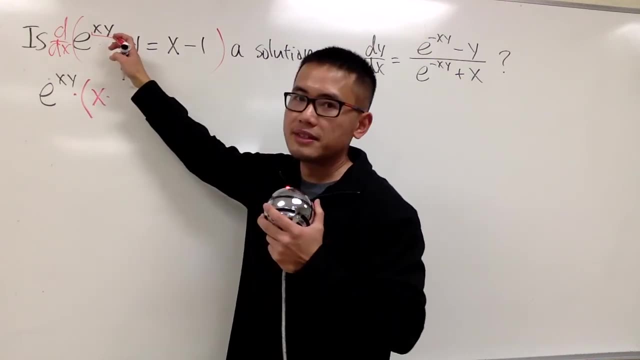 So I'll put this down in red. This is x times y. It's a product of two functions. The product rule says we have to keep the first function and we multiply by the derivative of the second. The derivative of y is just dy, dx. 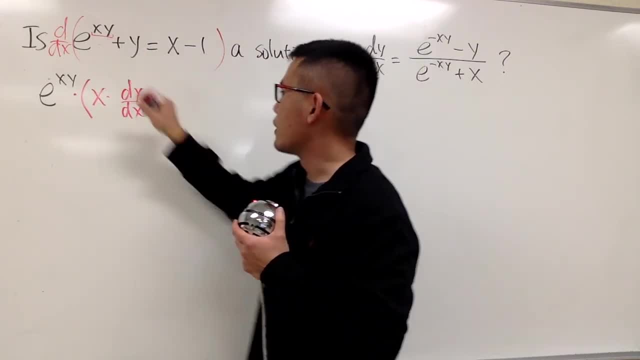 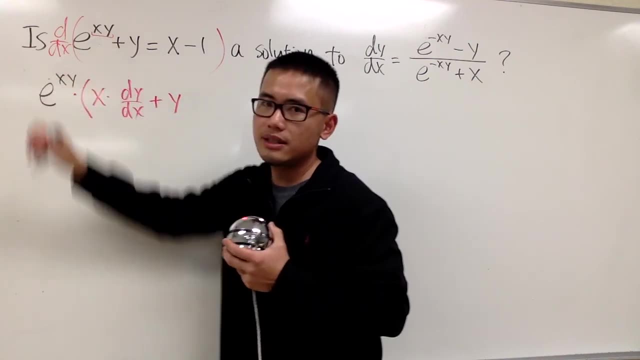 And then we are going to add the second function, which is y, and we multiply by the derivative of the first. The derivative of x with respect to x is just 1.. So this is just y times 1, like this: 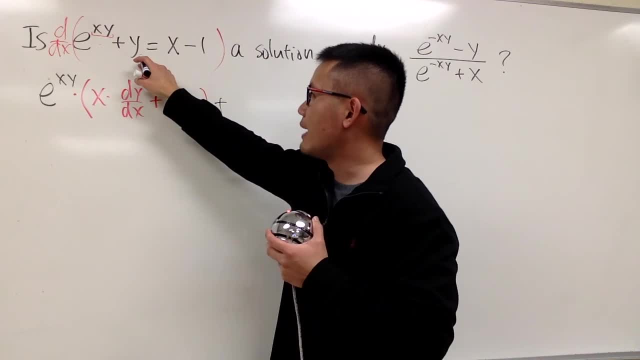 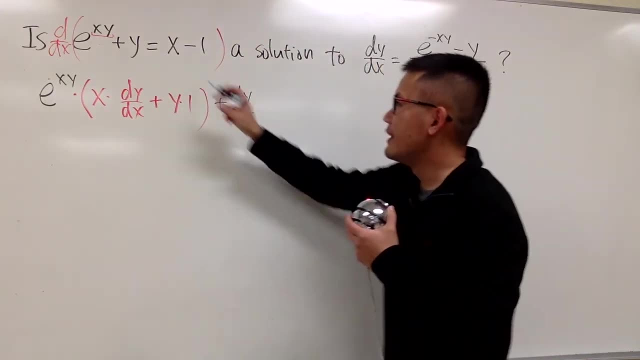 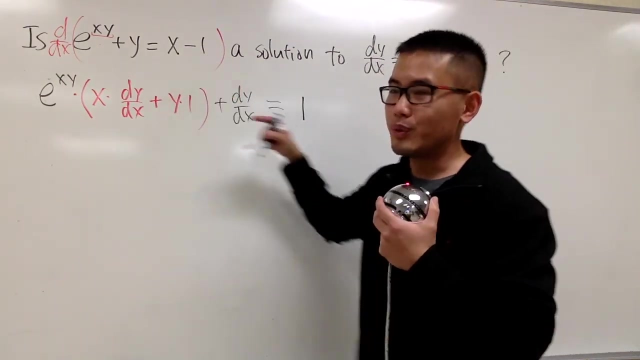 And next we add it with, we have: the derivative of y is just dy dx, The derivative of y is dy dx, and then we will have: this is equal to x. We take the derivative of that, it's just 1, and then negative 1, we get 0, and this is what we have. 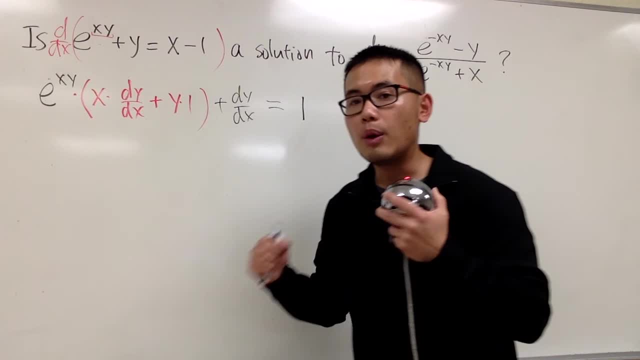 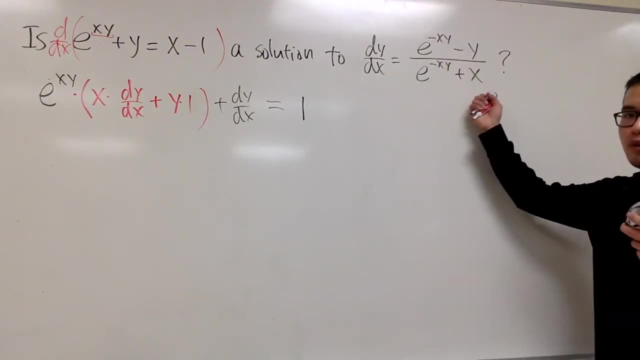 And now you see, we have the dy dx right here. right, Our goal now is to just isolate the dy dx, and hopefully that expression will be the same as the key from 1 right here. Well, let's do the usual business. 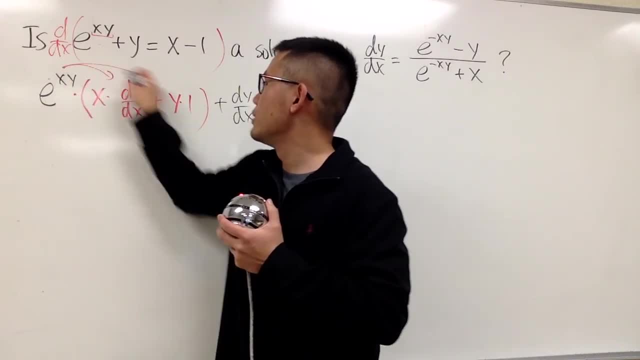 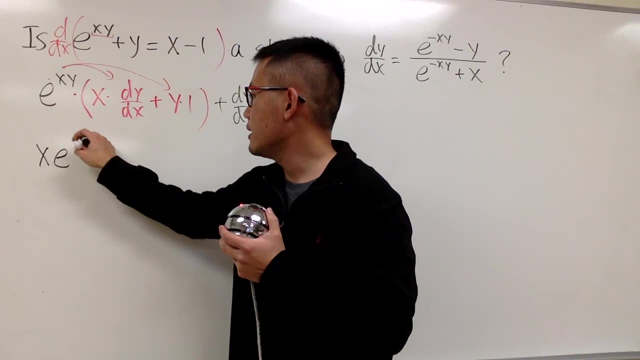 Here we have something in front of the parentheses, so we'll take this and distribute it into the parentheses. right? For the first part, we will write this down as x. So we have the dy dx e to the xy and then we have the dy dx. okay, 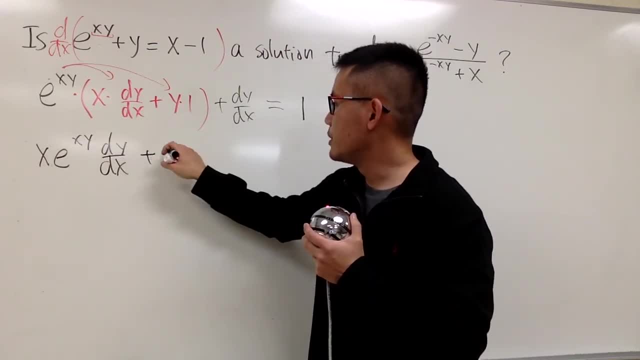 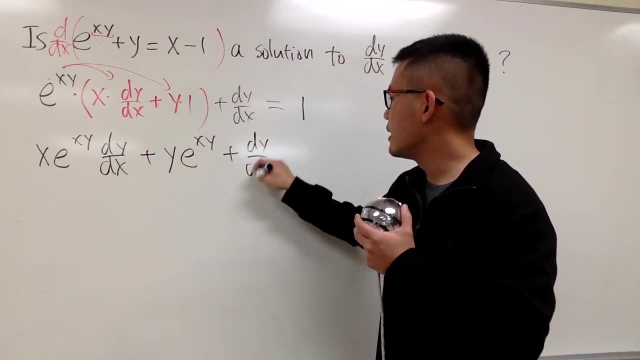 And then we will do this times that. so we add it with: let me put the y first, and we have the e to the xy, and then this is the dy dx, and then we have this: equals to 1.. Okay, here is the usual deal. 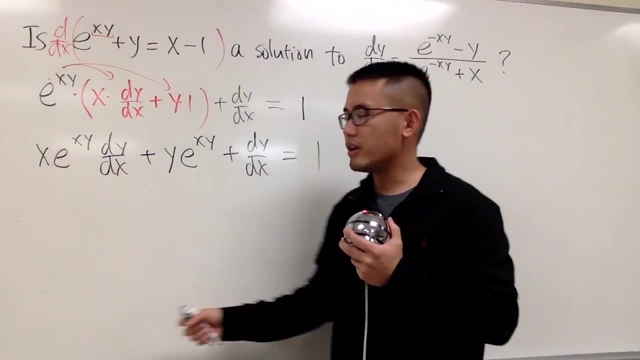 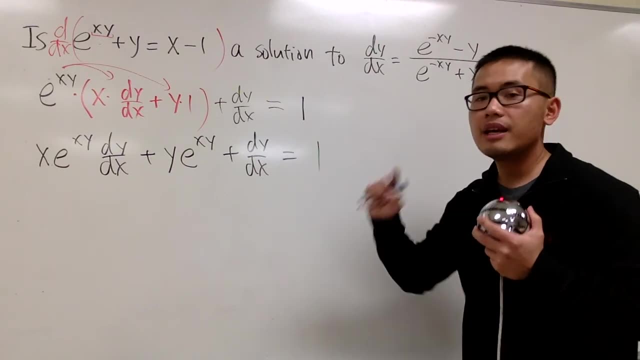 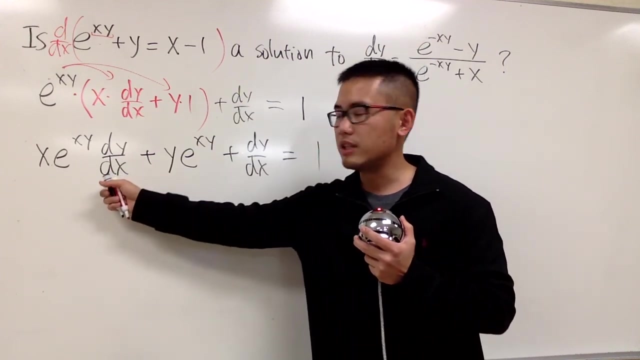 We have this expression now and you have the dy dx here and the dy dx here, right, But then I don't have the dy dx here. I'm going to move this to the right-hand side. In the meantime, I'm also going to keep both of this right here on the left-hand side and also factor out the dy dx. 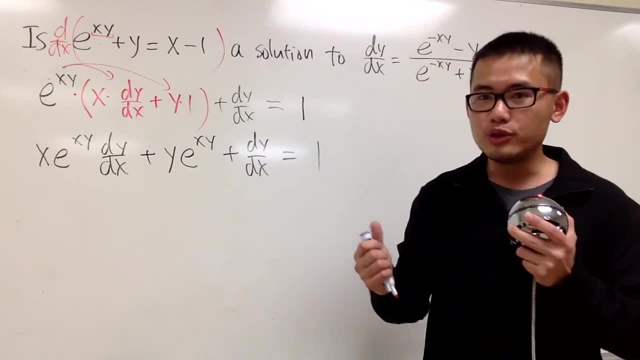 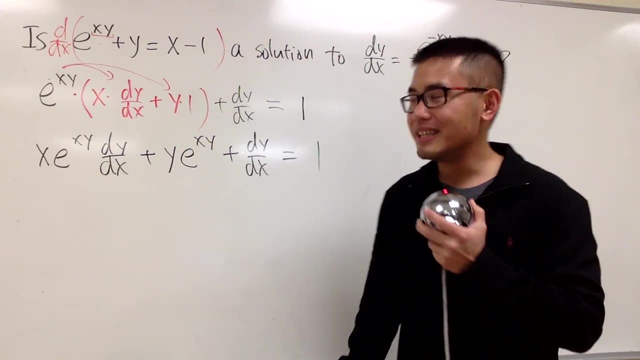 And to factor out the dy dx. when you're doing differential equations or things like this, put down the things, put down the dy dx at the end, because otherwise it seems like you have to differentiate again, right? So don't do that. 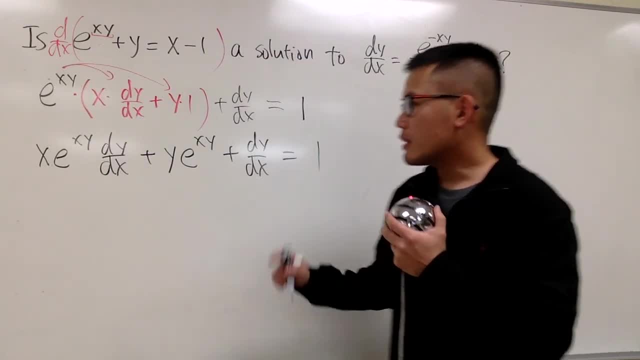 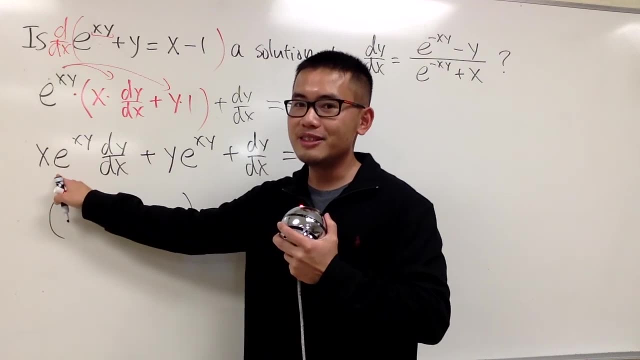 Put down the dy dx at the end. So let's do this carefully. I will open the parentheses. This right here has the dy dx and this is going to be the left over after you factor this out, right? Let me put this down first. 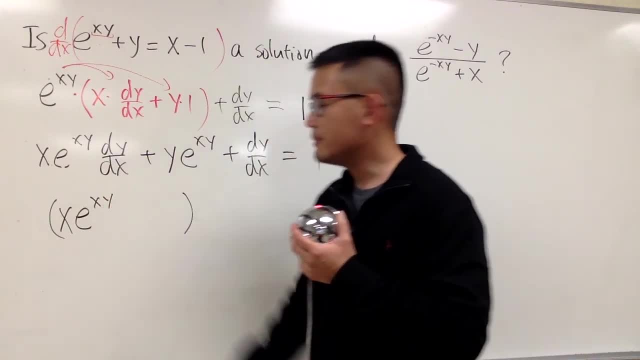 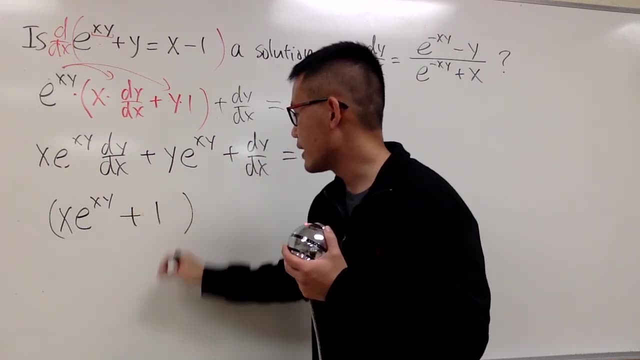 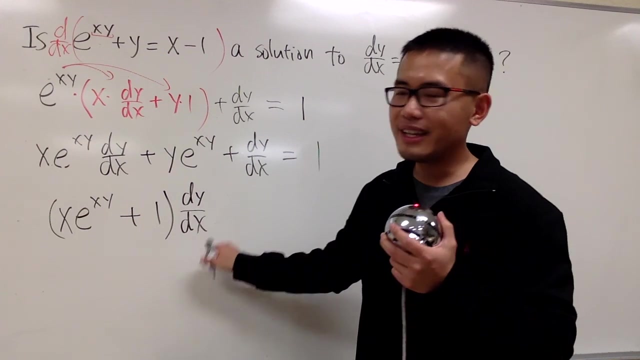 x, e to the xy, and this also has the dy dx and this is technically a 1, so it's a plus 1,. okay, And I will put down the dy dx at the end. Once again, write it down at the end. 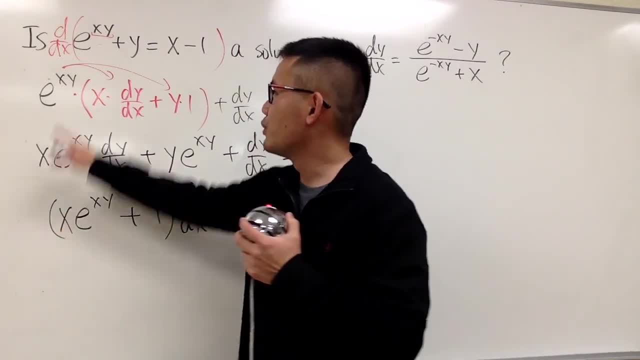 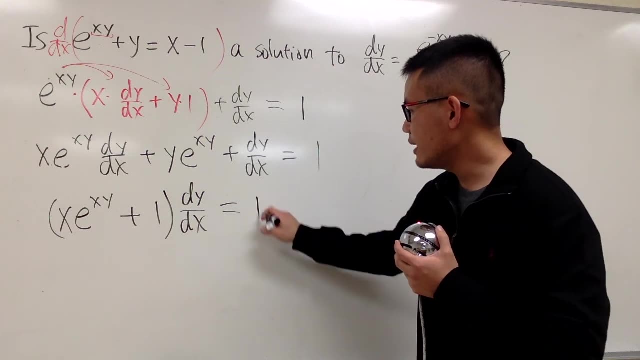 If you put it in the front, it seems like you have to differentiate again, right, So don't do that. This, I think, is more clear. Anyways, this is equal to the. 1 is still on the right-hand side, and I'm going to bring this to the right-hand side as well. 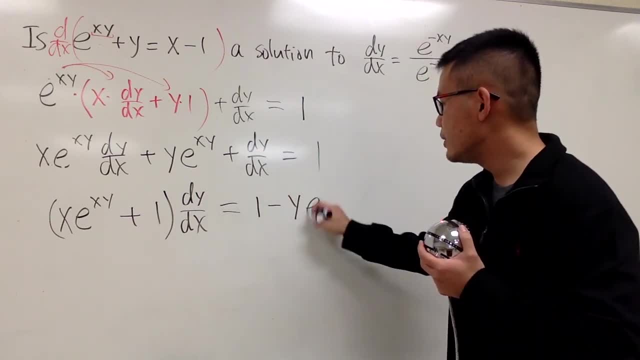 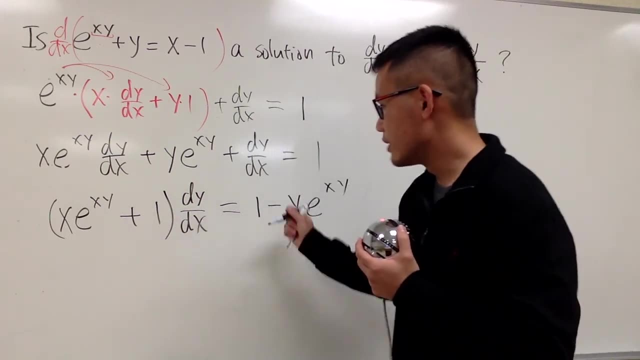 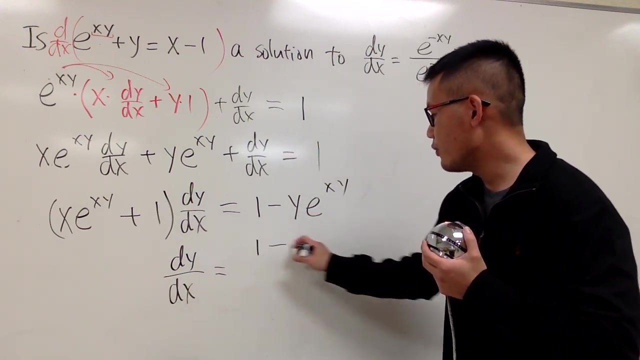 so it becomes minus y e to the xy, And now I can just divide both sides by that, isn't it? So, as you can see, we will have dy dx equals to this, which is 1. 1 minus y e to the xy over that. 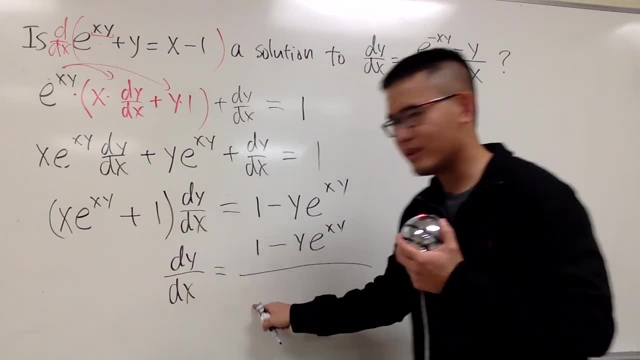 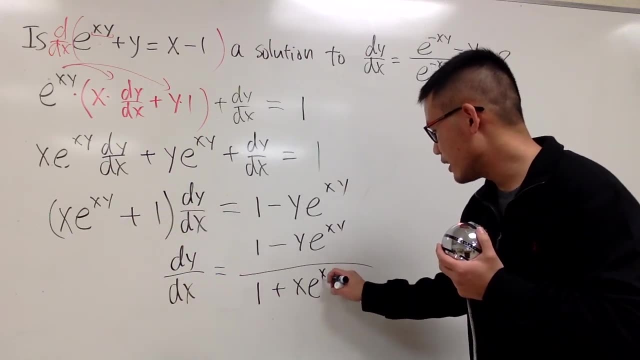 And since it has the 1,, let me put down the 1 right here. first, okay, 1, and then we add it with x: e to the xy. This is what we have, But this is what they give us.